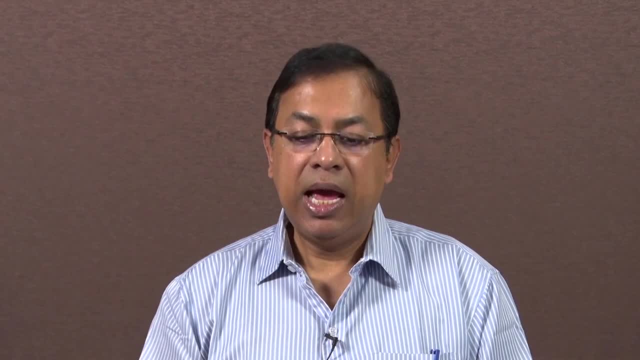 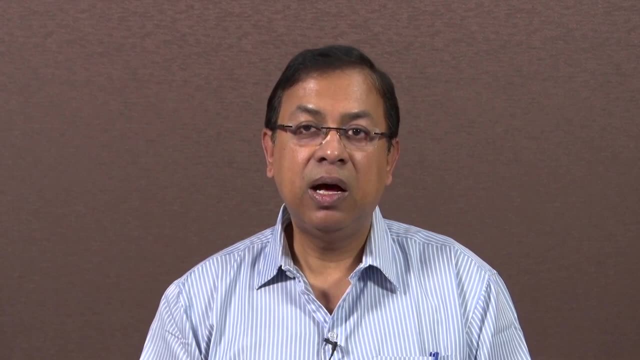 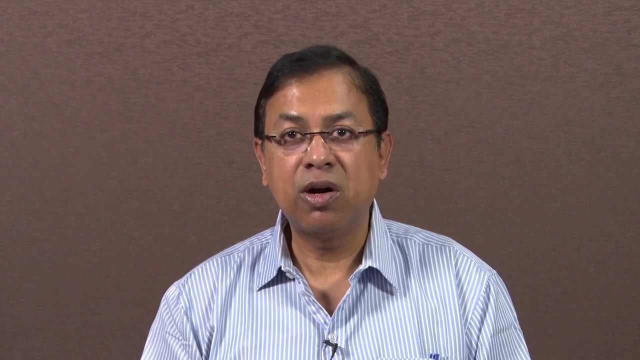 equal to 25.8 kilo ohms, And it's because of this reason that such an experiment, done in non-ideal conditions, can really give rise to the unit of resistance. in terms of the fundamental constant h and e was of huge importance, and 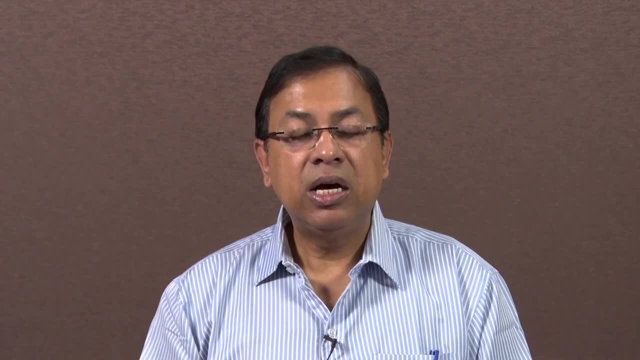 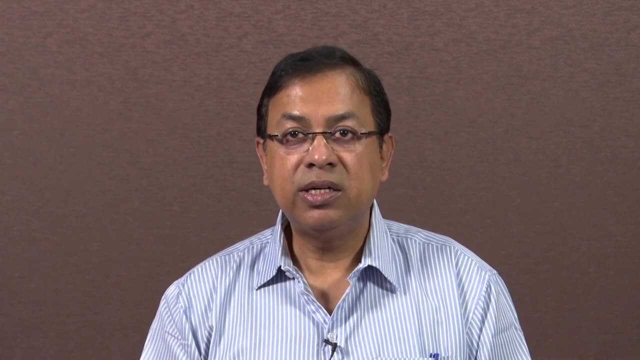 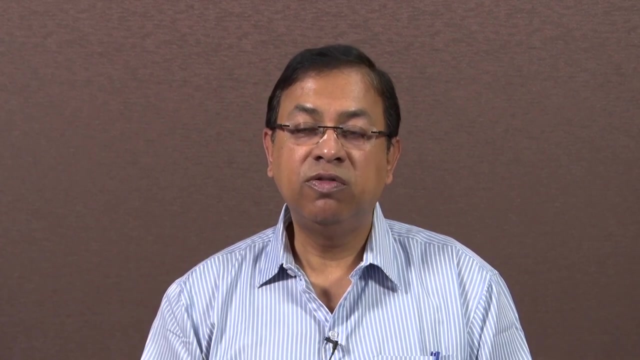 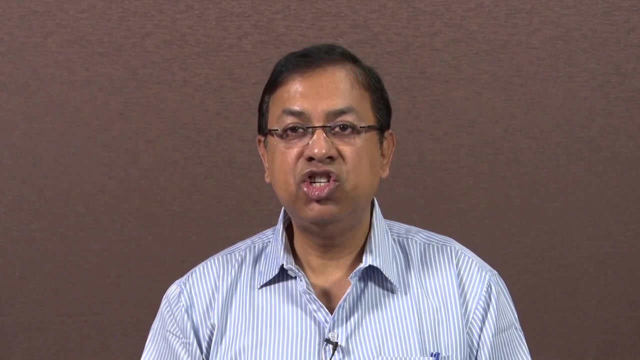 surprise to the community as well. This quantum hall system is also the first realization of a topological insulator. What I mean by that is that the edges are conducting and the bulk of the sample remains insulating. Now, this doesn't happen for an insulator, where both the bulk and the edge they behave similarly, But here the bulk. 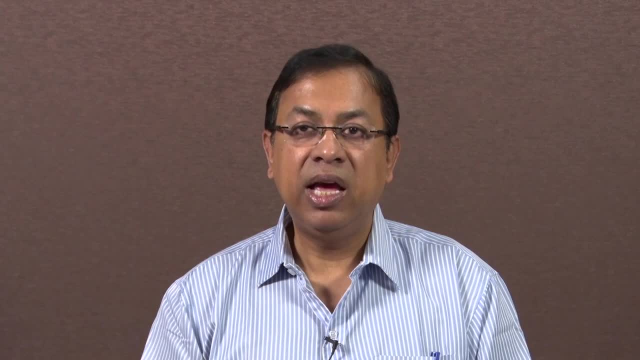 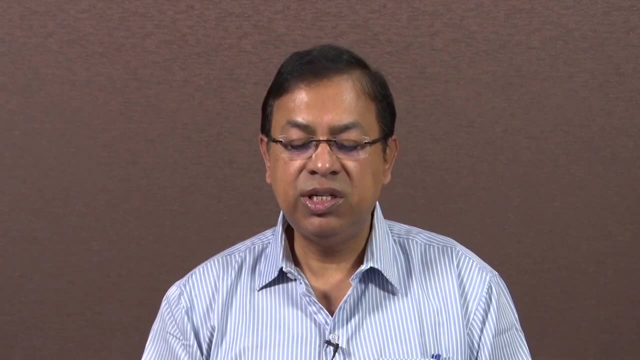 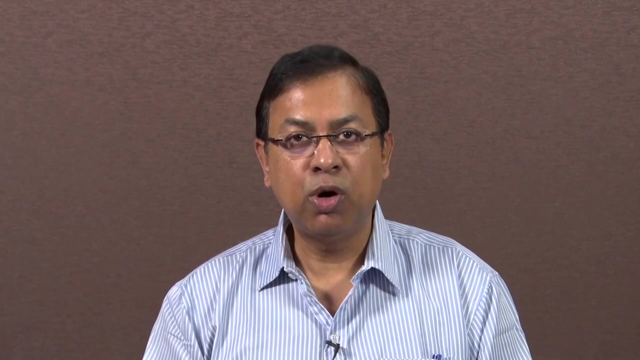 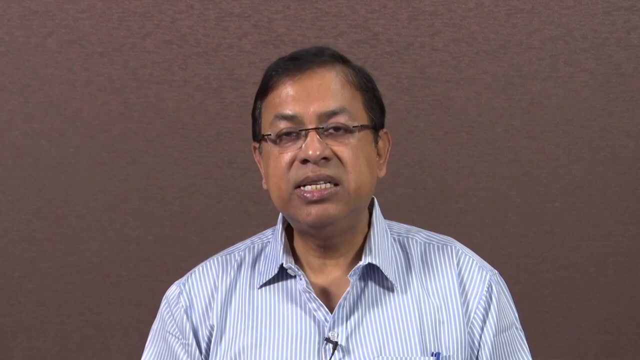 shows completely insulating behavior, whereas the edges remain metallic. In the course we shall learn how to compute Hall conductivity using Kubo formula and how the Hall conductivity is related to a topological invariant called as a Chern number, And to extend this quantum Hall effect in crystal lattices. we shall study this quantum 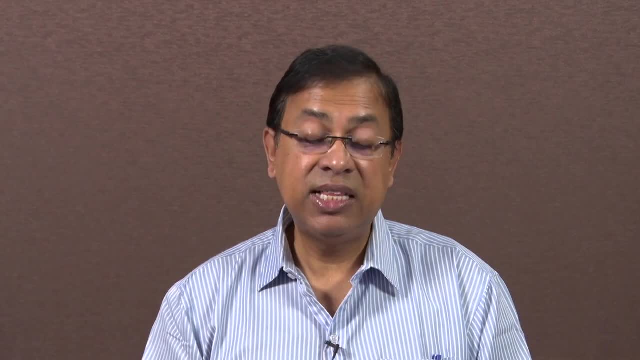 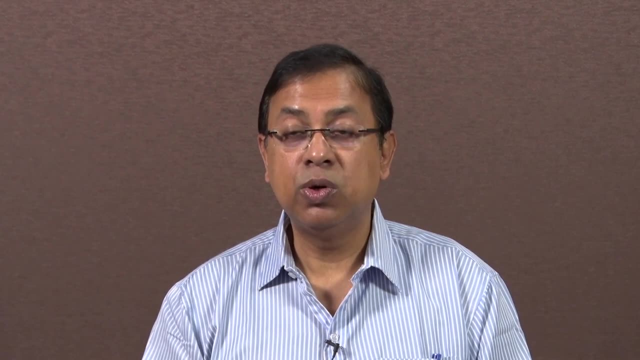 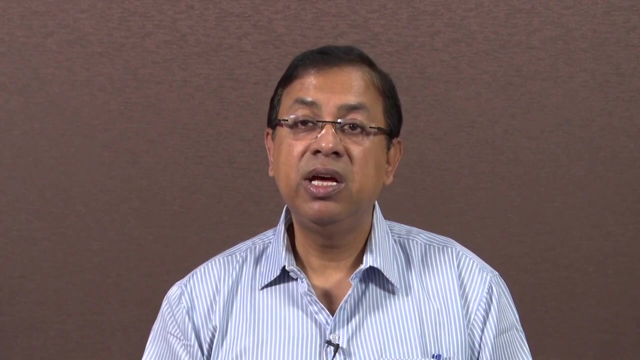 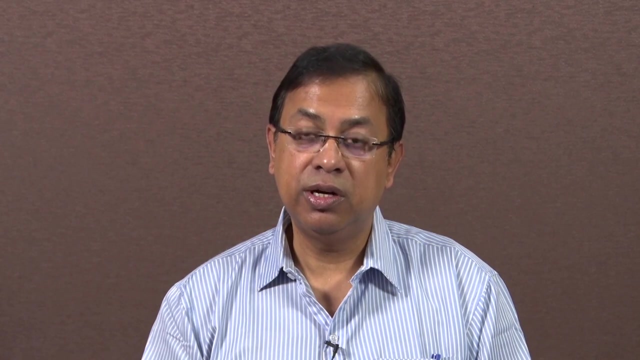 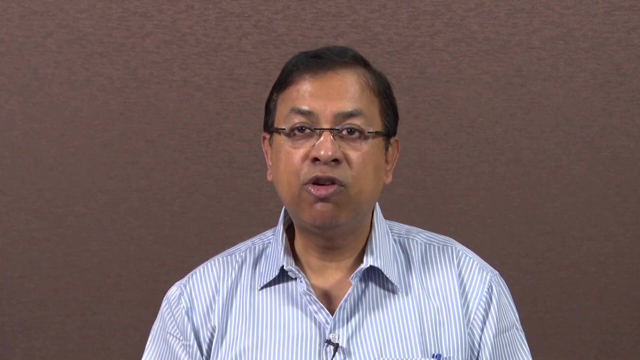 Hall effect in graphene, which said that the quantum Hall effect can actually be experienced at room temperature, because the difference between the energy levels in the quantum hall of these electrons in graphene and they show the energy scale, is of that of room temperature scale. And finally, we will study fractional quantum Hall effect, in which the electronic 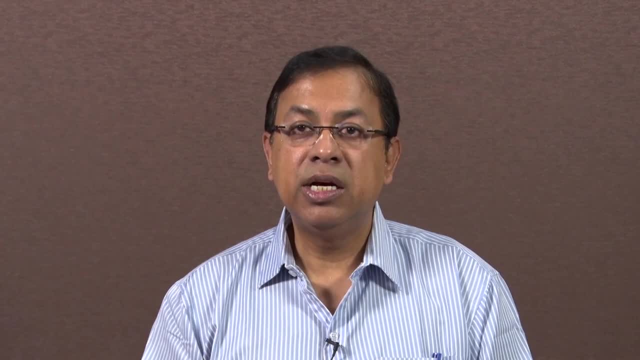 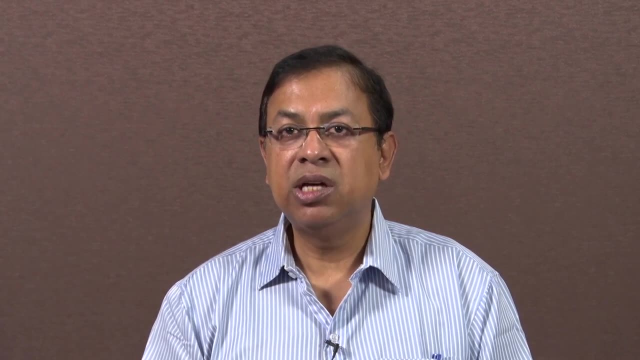 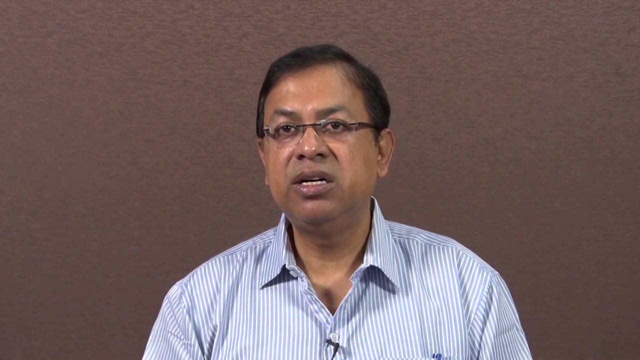 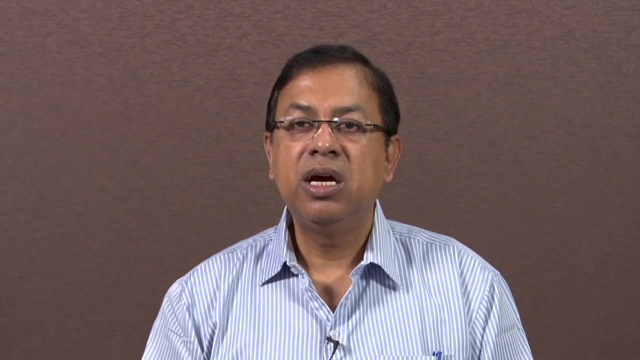 interactions need to be taken into account and these Landau levels being enormously degenerate, the coulomb interactions are indispensable and that gives rise to plateaus, not at integer times, h over e square, rather the integer actually leaves in the denominator, but it is also 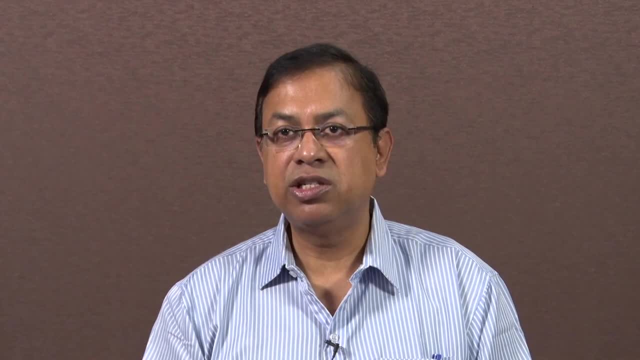 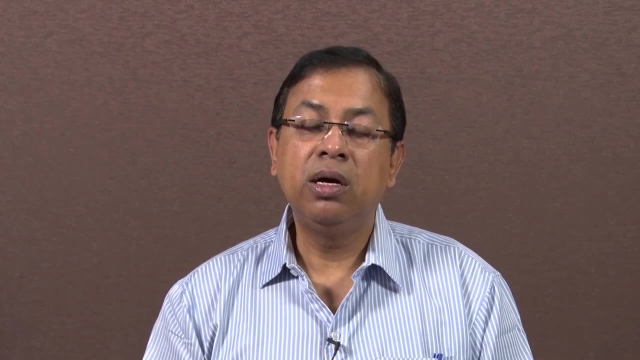 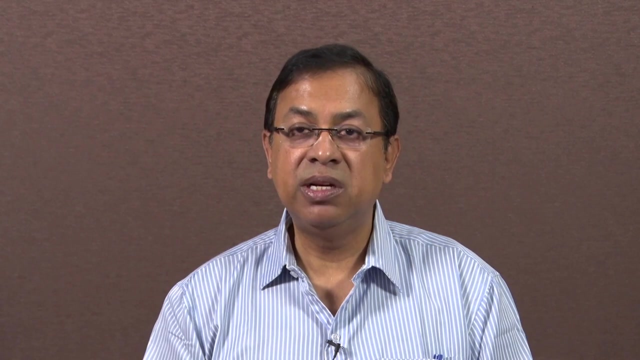 the in could be fractions as well and there are a large number of fractions being seen. and we will also look at spin Hall effect where the charge Hall conductance may be at absent but the spins actually segregate the up and the down spin segregate in transverse.